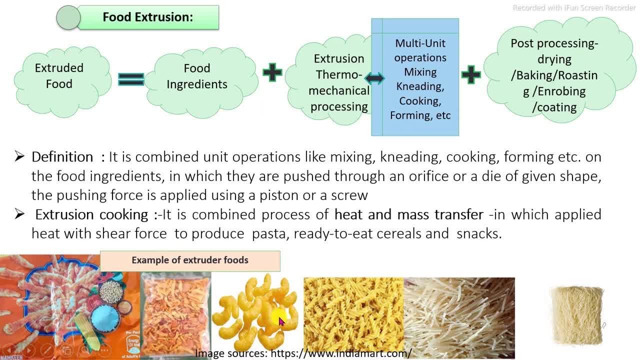 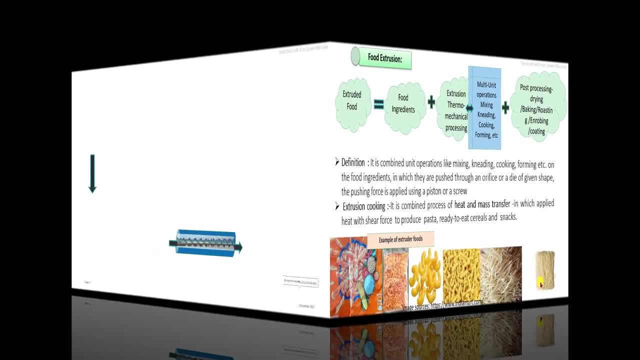 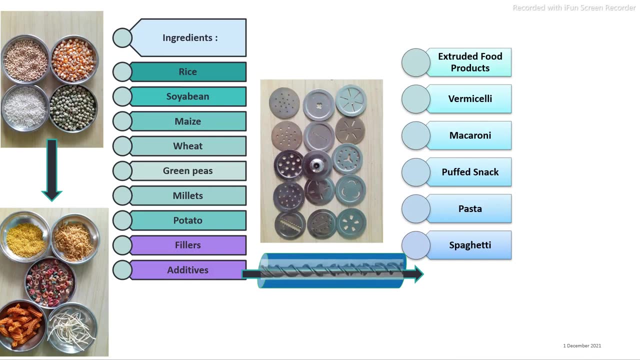 carried out and result in we get the number of products into the different shape size as per our requirement. In the food extrusion processing technology, the main raw materials for the production of the different extruded food products, In which the main basically raw materials based on the cereal grain with added maybe. 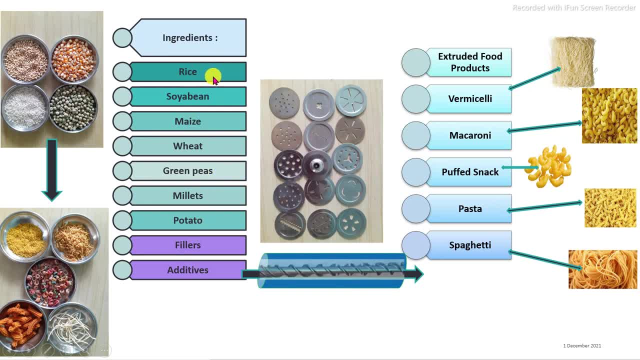 pulses, oilseeds, potatoes are the main raw materials which are coarsely milled and used for the production of the different extruded food products. preparation along with the addition of the number of the additives in which, basically, these raw materials are first milled into. 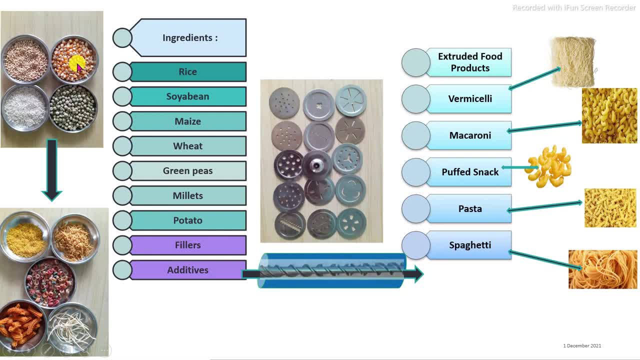 the coarse milling, or maybe sometime used as a directly for the extruded products, like the puffed product preparations in which these raw materials are converted into the final product by using the extrusion technology in which product is passed through the. by providing the dyes as per our requirement, they can convert into the different products. 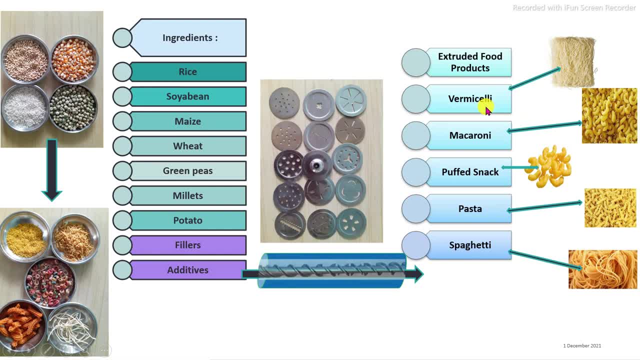 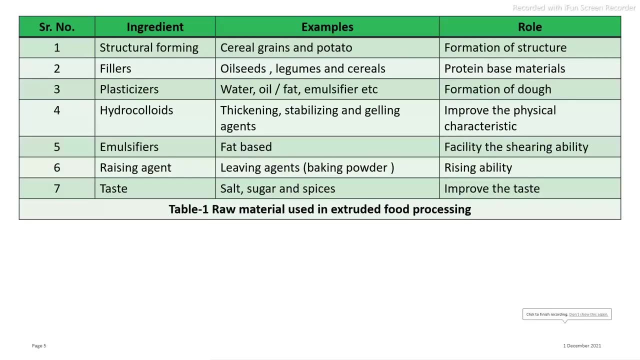 The main product involving that is the first one- is the vermicelli, in which snacks pasta processing, then spaghettis. these are the number of the product which are prepared in different shape and the size by the extrusion technology. The raw material used for the processing of the extruded food processing in which the 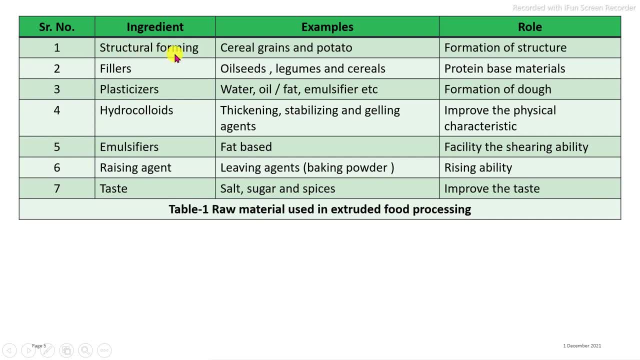 main raw material. that is, the first one is the structural forming raw material, in which cereal grains and the potato main, which is forming from the final structure of the potato, of the product, then fillers, in which the oil seeds legumes and the some of the cereals. 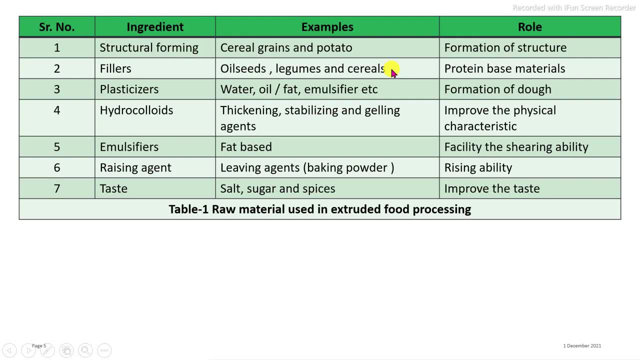 which are added, which are the protein base to, in order to control the puffing of the final product. then plasticizing ingredients, in which the water, oil, fat, even spaghetti, which is helped to formation of the dough, and facility for the smoothening of the final 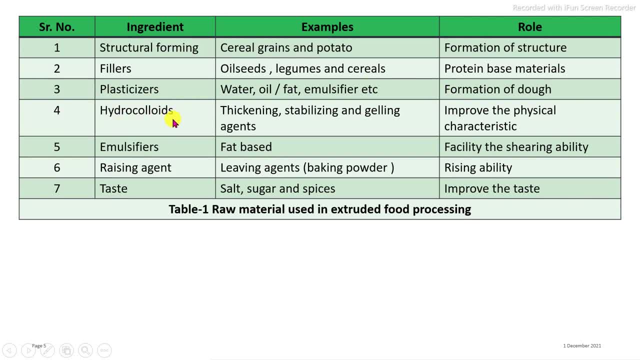 product. Then hydrocolloids, material in which the thickening, stacking and compaction of the final product. This is the structure of the final product and this is the material used for the final product. stabilizing and the gelling agents: these are the additives also added for the specific. 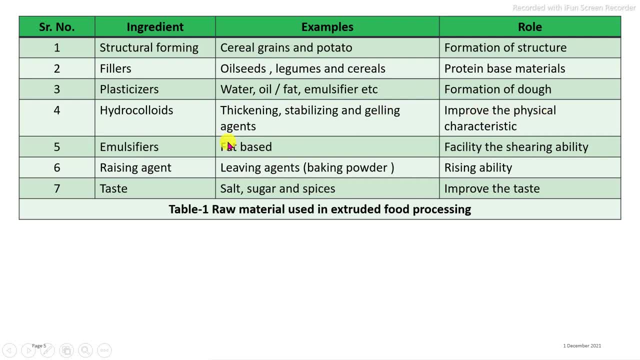 improving the physical property of the final product. emulsifying agents are added on the base of the fat dissolving, that is, the fat base. emulsifying agents to facilitate smoothening for the shearing ability. then rising agents, that means the livening agents in which the 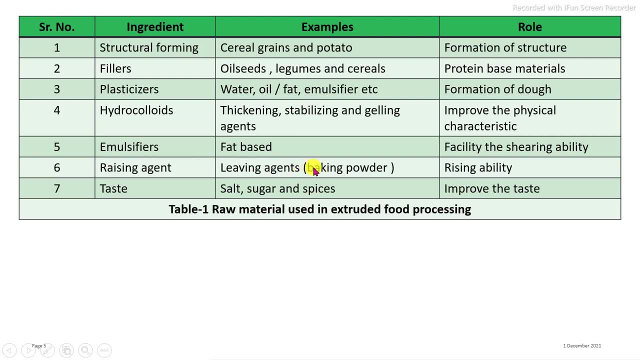 baking powder is mostly used as a livening agent for a specific baked product- which are extruded, then taste improving agents, in which the sugar, salt and the spices which are added in order to improve the taste of the final product. these are the main ingredients, examples and the 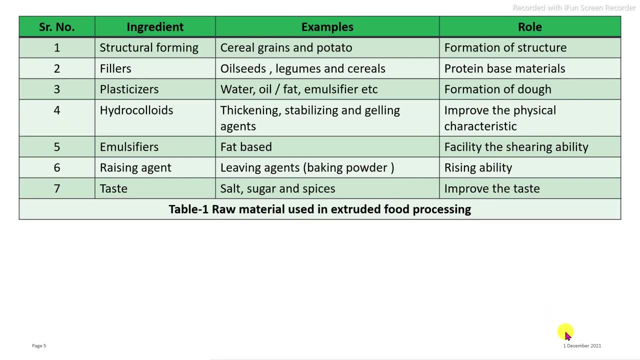 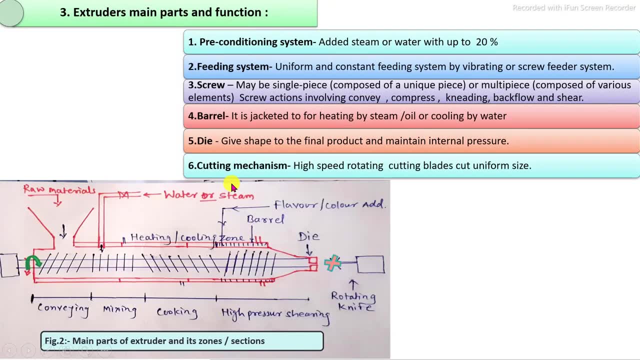 role of the ingredients in the extruded food processing. the main parts of the extrusion machine, in which the main parts involving first, that is, the extruder screw which is fitted at the center of the barrel- this is the single screw extrusion in which internal of that barrel centrally mounted. 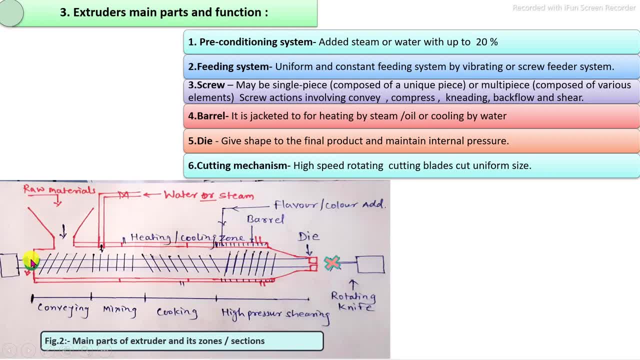 screw, there should be the provision of the provided with the bearing systems, then provided with the pulley and connected with the power transmission devices. so the barrel externally fitted with the steam jacket kettles in which the heating and cooling system. heating and cooling system is carried out by circulating the steam through the external. 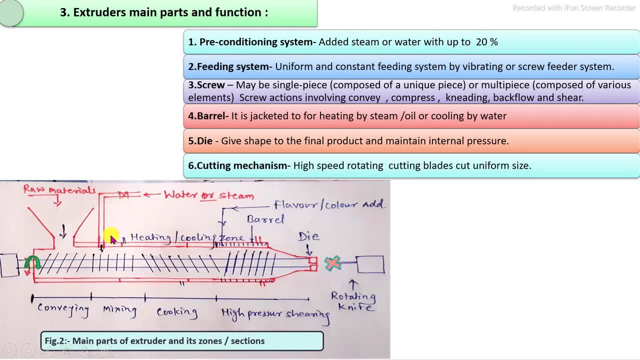 jackets. then there should be the provision of the feeding of the raw material from the hopper into the this extrusion machines. the feeding of the raw material is carried out by using the screw conveyor systems or the vibrating system in between. they are the intermediate addition of the liquid ingredients, like the chunk of water. 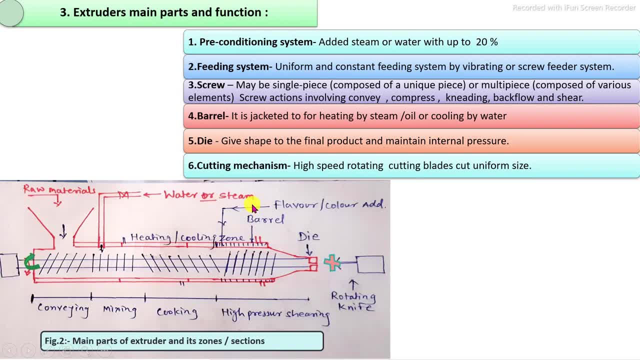 or may be: addition of the steam or the oil, addition and flavoring substances. the main screw which is divided into the components using the conveying section, mixing section, cooking section, high pressure sharing section and, finally, forming section, which is the Grayning poor kitchen. this is a competing 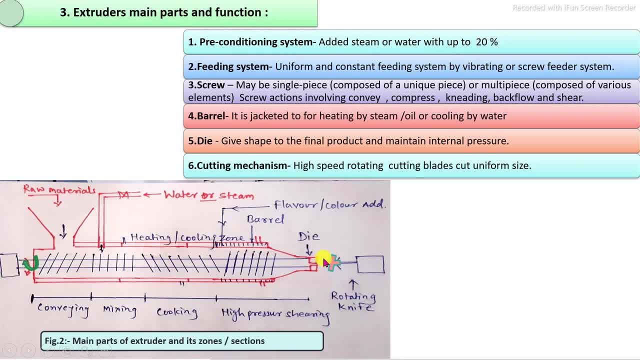 where the the dust accumulates, will be generated by cheese commission and gegeben as a dropper, resulting in the change as the liquid farminases. this will help in Syrup, in fact, by boiling, separation of LCD or contaminated at the water, new groundwork, peạnh, comfort, master or green building system. 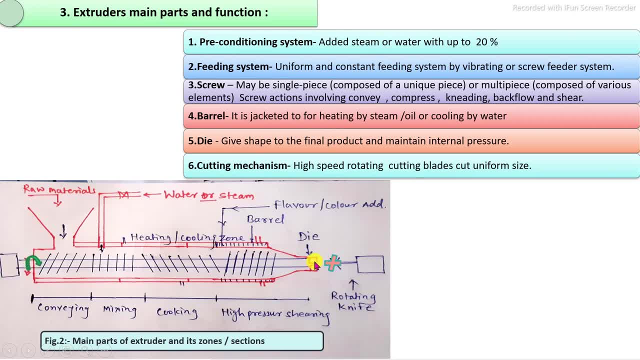 well, first- this is a favorites edit- under the, there should be the provision of the dye, which is theBLE intermediate jets. this is the water diluted well, and normally we will secure fresh, finished, collected into the water. gesagt change as per our requirement. and finally, the rotating knife. that is the cutting mechanism. 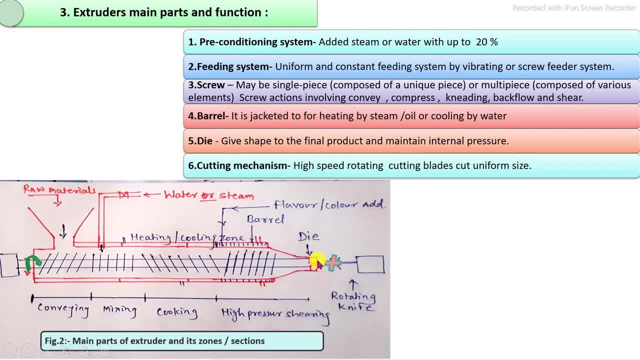 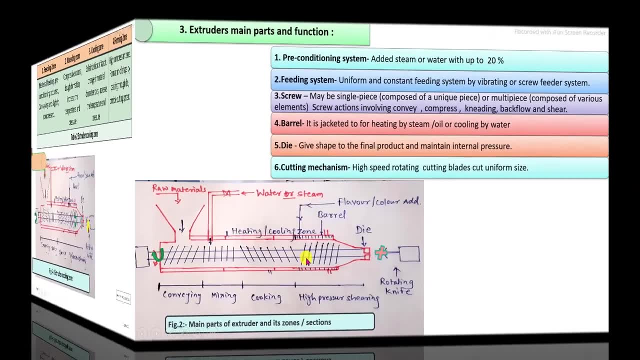 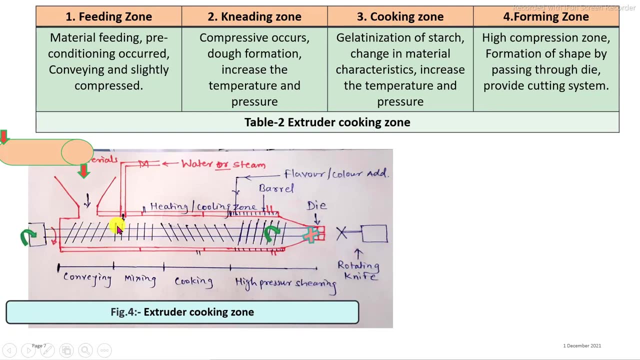 after the extrusion of the product, which is cut into the different size as per our requirement. these are the main parts involving in the extrusion machines. in the extrusion machines, the extrusion machines are specifically sections, or also called as a zone in which the feeding zone, kneading zone, cooking zone and the forming. these are the basic zones. 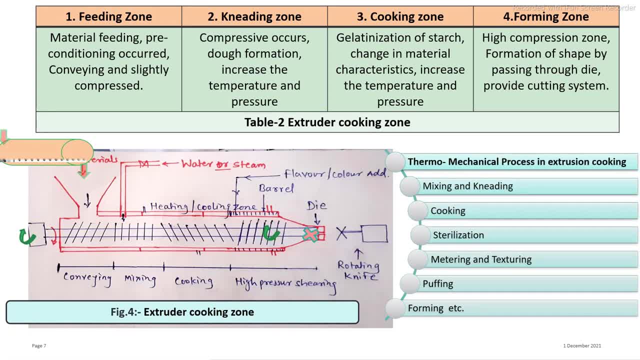 in the extrusion processing technology, the materials which are first pre-conditioning is carried out or may be pre-conditioning, which is provided in the extrusion machine. also, the dried metals are loaded by providing the feeding system, by using the screw conveyors or by using the 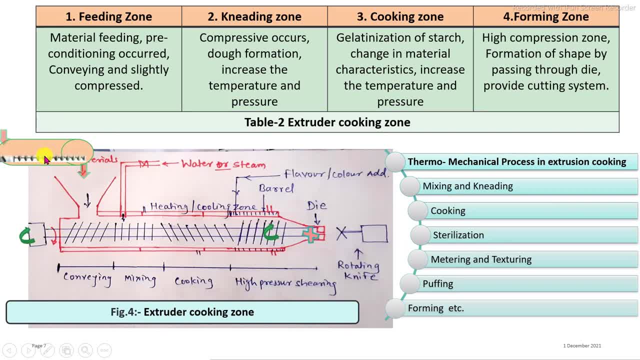 vibrating devices in which the materials are continuously, uniformly, with constant rate, feeded into the extrusion machines. after the feeding of that material- the first the materials are first pre-conditioning- is carried out into the feeding sections. first they are pre-conditioning with the addition of the steam and water and other whatever the liquid ingredients, and after that. 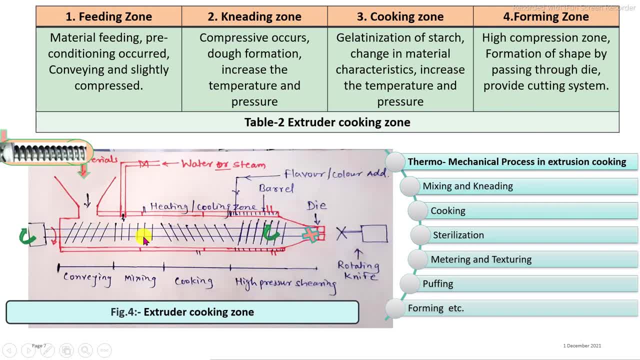 mixing, pre-mixings and the final mixing, in which the final mixing, kneading is carried out, in which the slightly pressure is increased and the formation of the dough, which also increasing the slightly temperature and the pressure in the mixing zone. after that, the next one is the cooking zone. there. 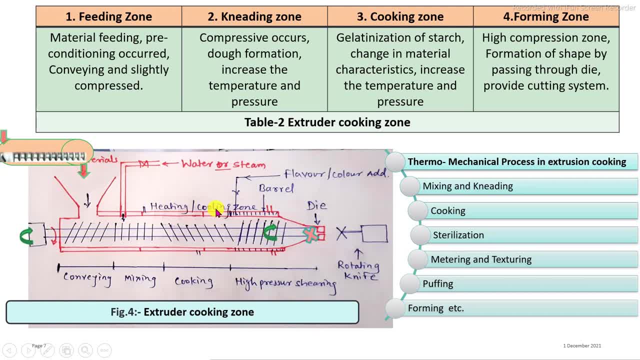 should be the provision of the external jacket to circulate the steam or some extruder provided with the electrical heater systems. in cooking zone the gelatinization of the starch is carried out and after that the cooking addition of the flavoring and the coloring matters in liquid form. 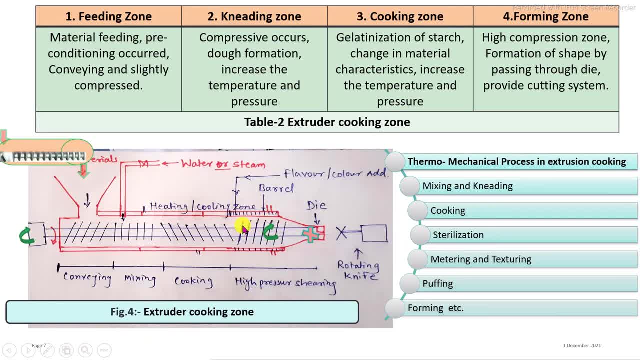 then next one is the high pressure sharing force and last one is the forming zone. forming zone in which the compressor and pass the water, the which is prepared, into the specific provided with the dye, and finally cutting this occur. these are the main zones involving in the extrusion machines. 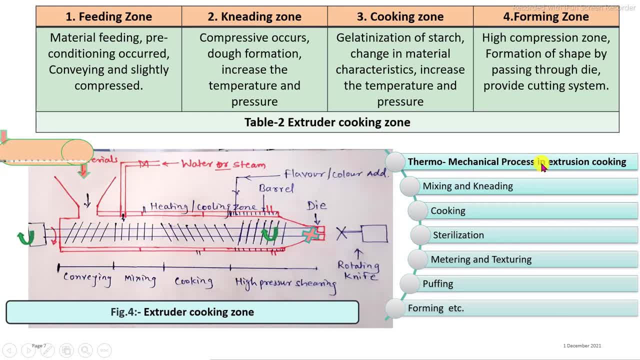 in the thermo mechanism process, in the extrusion process involving mixing, kneading, cooking, sterilization, then mattering and the texturing copying forming. these are the various unit operations which are involving in a single extrusion machine. the extrusion machine screw may be either a single 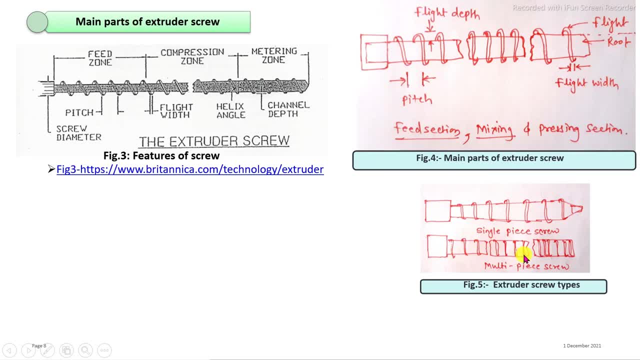 piece or maybe into the multi piece screw system, single piece in which the mostly tapered shape which is used for in cold extrusion is also used as a whole machine yr process. and in multi-piece system there should be that they are divided into the sections and most is for the hot extrusion process. the main parts of those 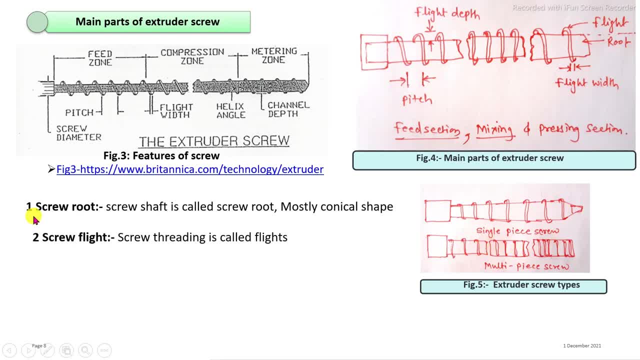 this screw is. first, one is the screw root. that means the root, that is the screw shaft is called as a screw root. that means the total shaft of that. a screw is called as a root, mostly in a conical shape, that is the tapered in shape and specifically on the top of that root, provided with the flights, the 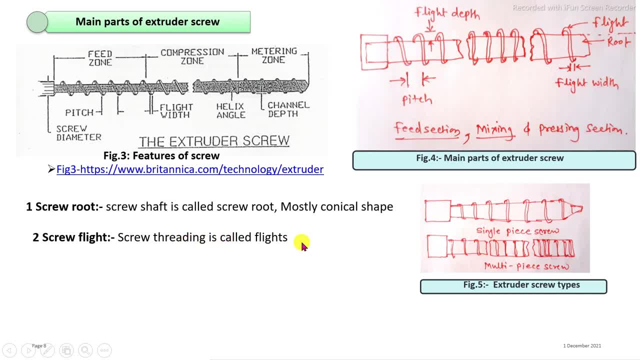 screw flights that mean the screw threading is called as a flights then pitch. that means the distance between the flights. nearest flight distance is called as a pitch, and flight distance is called as a pitch and flight depth. that is the. this is the width of the flight and this is the depth of the. 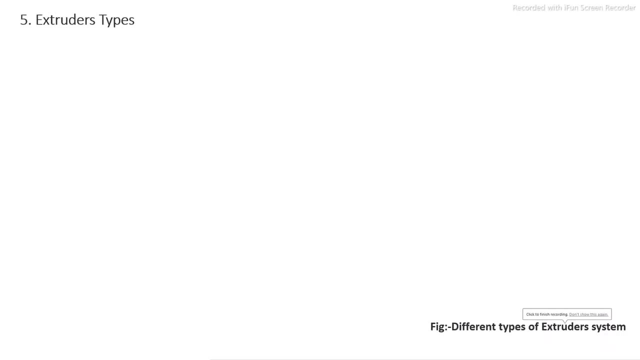 flight. the basic types of the extrusion system with, on the basis of the method of operations- cold extrusion, hot extrusion system- and on the basis of their internal provided single screw extruder, or may be provided with the twin screw extruders. different type of extruders are: the extrusion system with extension. 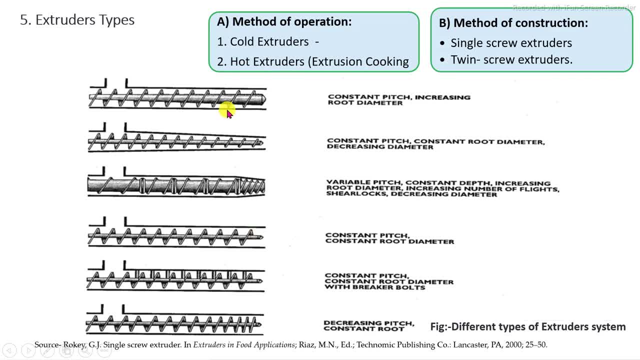 of the extrusion systems in which, basically, these are the number of the systems in which the specific designs, in which variation of the root diameter with respect to the length of that extrusion machines, or change of the diameter of the barrels with respect to the length of the extruders, then variable pitch with respect to the length of the extruders. 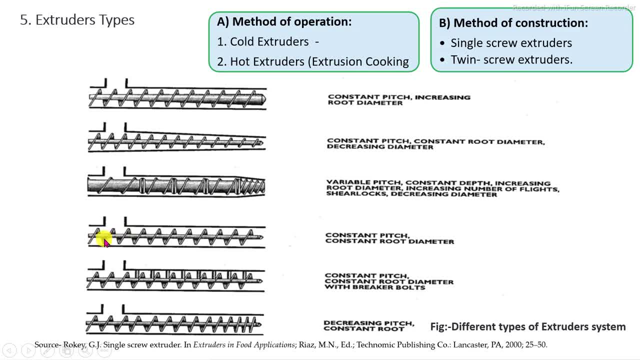 then constant pitch, constant root and the constant diameter of the extruders, in which internally provided bolts, in which the bolts which produce the more shearing force, then in which the pitch distance is variable, with constant diameter of that extruders. in this way, number of the designs are available for the extrusion processing. 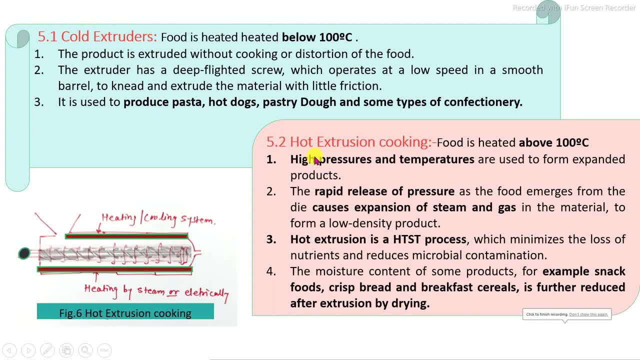 The basic difference between the cold extrusion and the hot extrusion technology is that cold extrusion that means what is heated or which is the extruded below 100 degree Celsius temperature, and the hot extrusion system internal temperature is more than 100 degree Celsius in the cold. 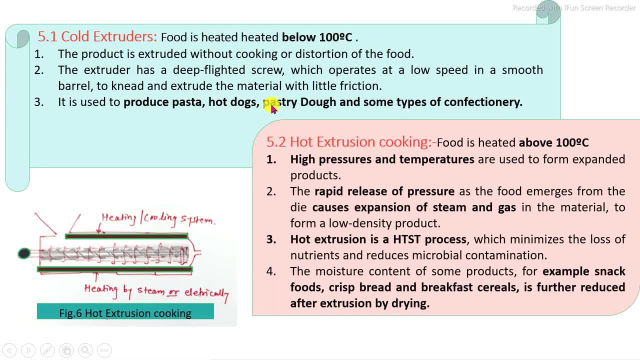 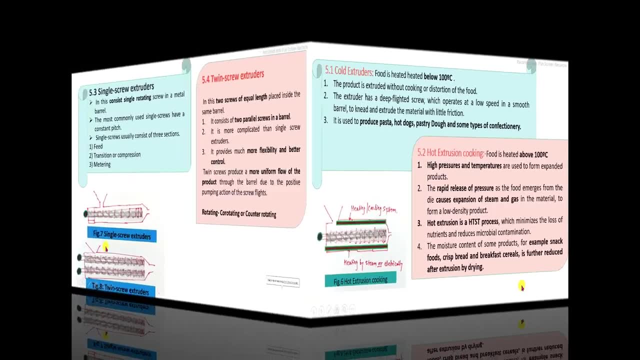 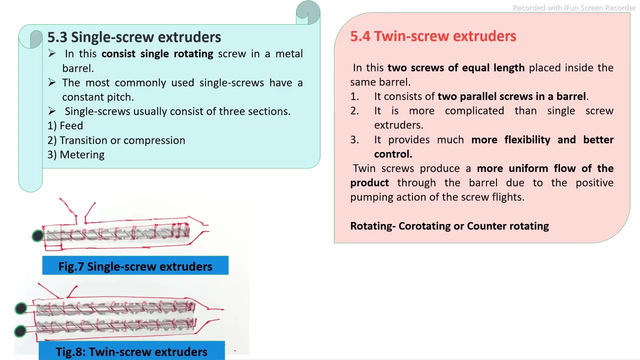 extrusion technology, mostly production of the pasta related product, model related products, which are the prepared and the hot extrusion processing, in which the puffing products are or the ready to eat products or the snacks, which are the prepared by the hot extrusion technology, The single screw extruder and the twin screw extruders, as per our requirement. internal. 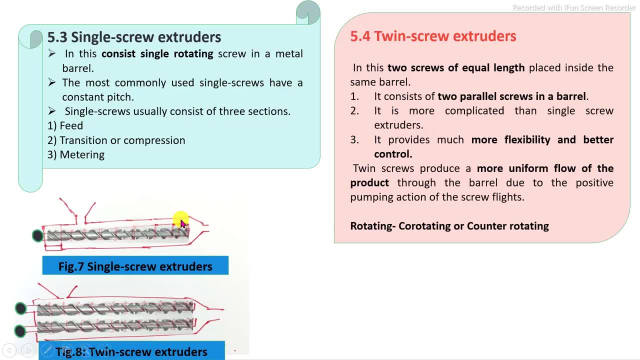 shearing force or the specific type of the ingredients and the final product requirement. we can use the single screw extruder or by using twin screw extruders. mostly single screw extruder used for the production of the pasta and noddle related products and the twin screw. 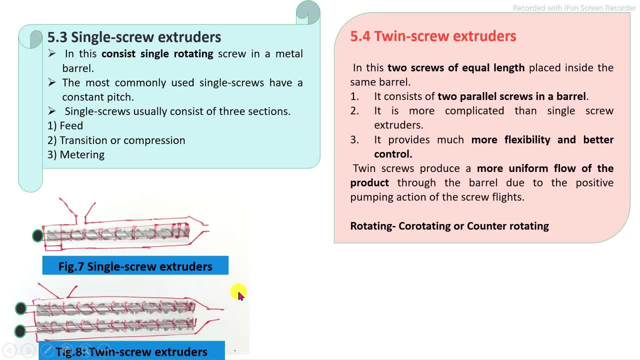 extruder used for the more shearing force in which the maybe operated co-current and counter current rotating extruders in which produce the more shearing force as compared to single screw extruders and prepared the different type of the extruded food products. 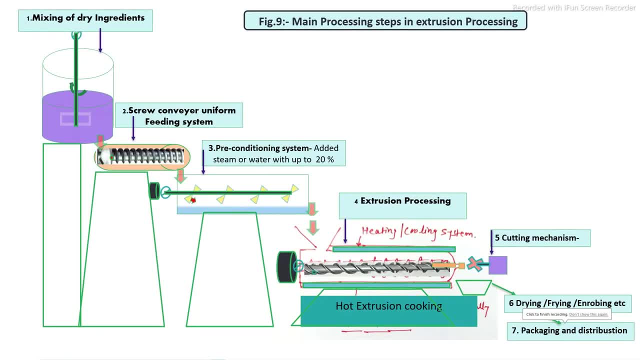 The main steps involving in the processing technology of the extruded food products. at the first is the mixing tank, in which the dry ingredients are first properly mixed up. whatever the cereal grain grids, the different type of the cereal grain grids with added with the, whatever the dry ingredients, these are the properly first mixed. 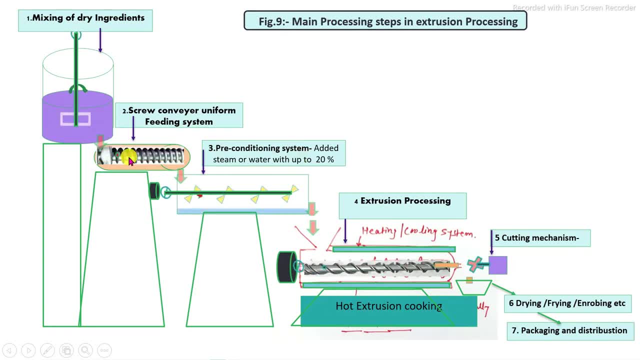 then feed into the preconditioning system by providing with the screw conveyor feeding systems in the preconditioning systems, addition of the waters or maybe addition of the steam injection or addition of the oils and other nutrients, or maybe added with the additive substances in this preconditioning system, premix. after that premix, which is the loaded with the screw conveyor system into the continuous extruder machines. 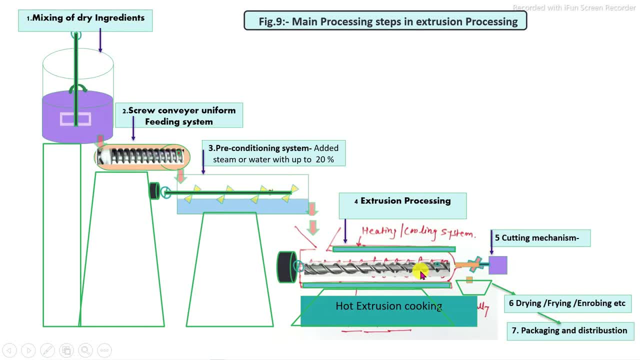 in this extrusion machines system to produce the extruded food product. after that the cutting is carried out and finally they may be dried, fried or maybe coated, and finally they are packed. these are the main steps involving in the processing of the extruded food product preparation. 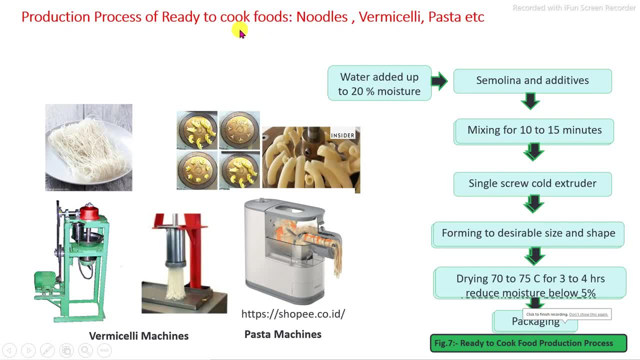 the production process of the ready to cook products, in which the noodles, vermicelli pasta product. these are the products which is prepared by the extrusion technology, the vermicelli making machines, which is operated by the electrical motor. this is the hand operated vermicelli machines or maybe number of the machines are available. 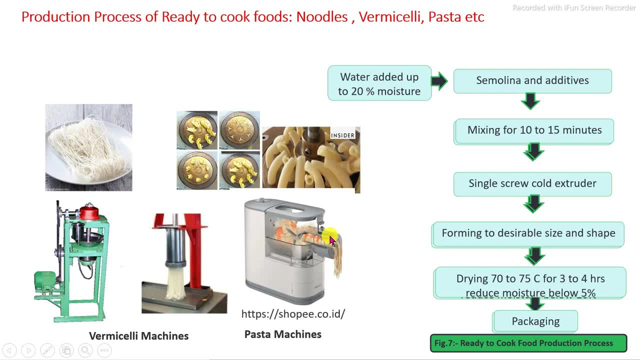 in which the pasta and noodles are automatically. we can prepared by only simply. we can change the dye as per our requirement. we can convert the raw material to the different shape, size of the noodles, vermicelli and the pasta product. it is the main steps involving first ingredients, in which the semolina 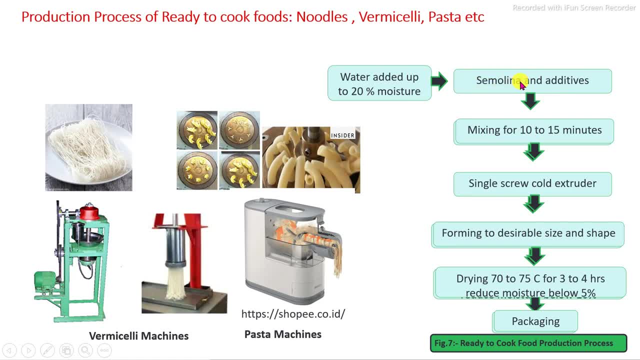 the semolina mostly used for the durum beets. durum beets with added with the some of the additives and added with the moisture, that is, the water is added to increase the moisture percentage up to 20%. then first they are preconditioning with addition of the water. 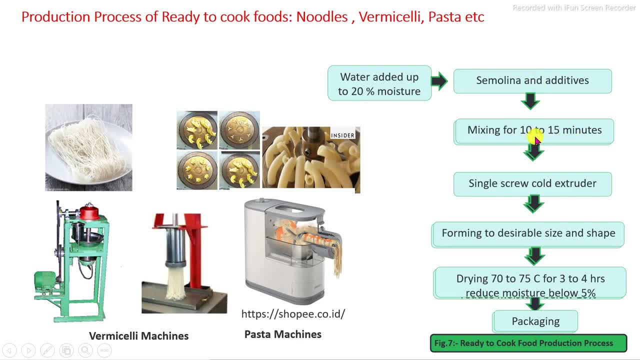 then are properly mixing for the 10 to 15 minutes, then processed into the single screw extruders to formation of the shape as per the noodles, vermicelli and pasta products, and finally they are dried to reduce the moisture content up to 3 to 4%.